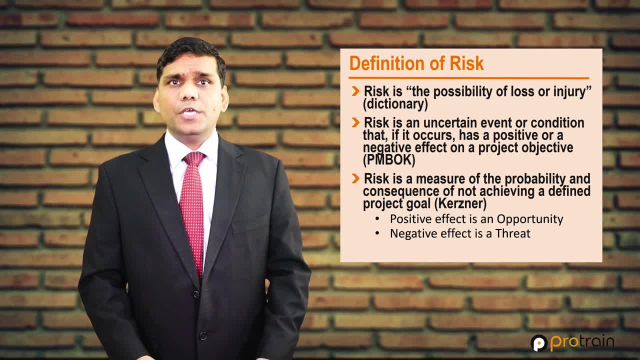 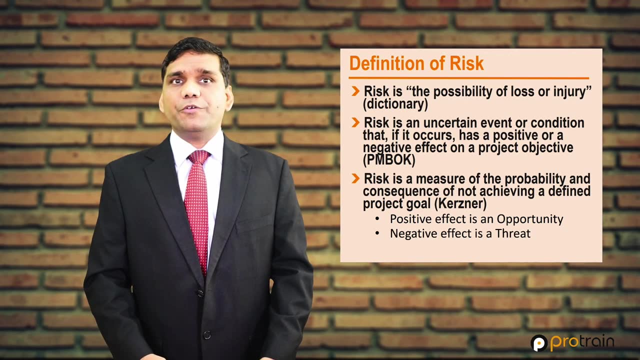 and negative risks are threats. Positive risk is almost a philosophical thing. It is all in how you look at it. Many people are convinced it does not exist at all. Other thinks of positive risk as an opportunity. For example, a project has US dollar 10 million. 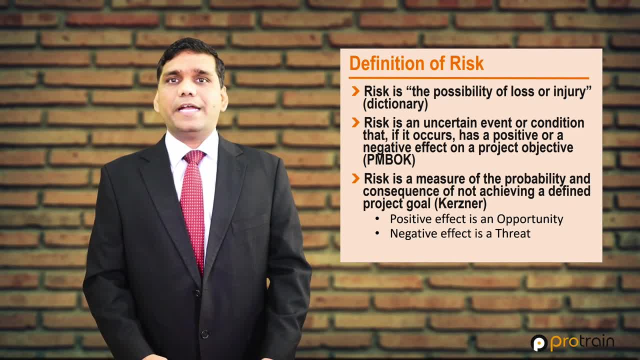 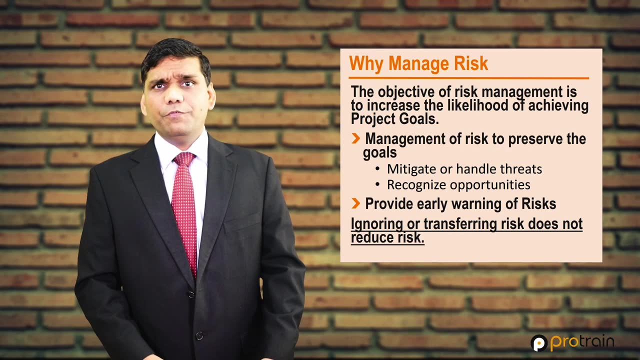 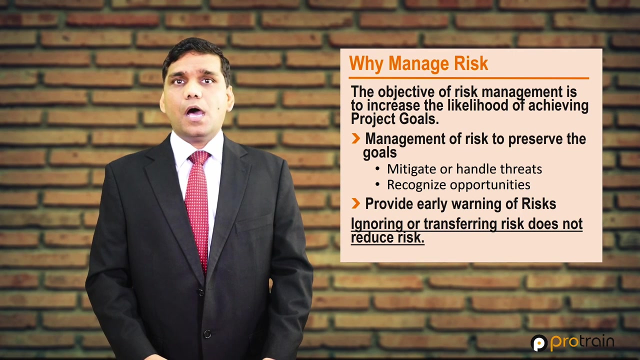 early completion bonus. Planning engineer determines that by augmentation of resources costing around US dollar 2 million, early completion can be achieved. This is an opportunity or positive risk. We need to care about risk which may turn into problems. Also, we can reduce or avoid future problems. 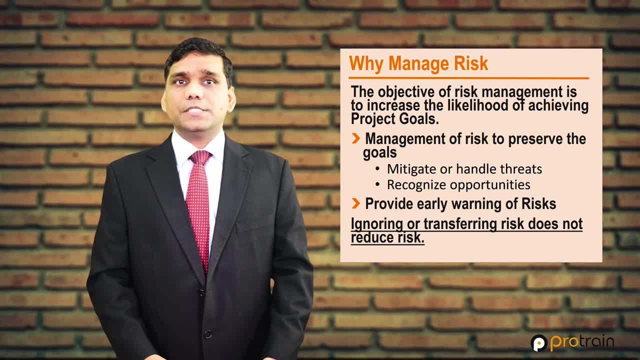 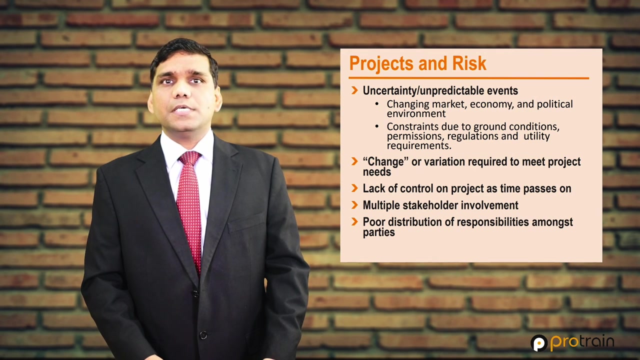 by reducing their consequences or their probabilities. If risk is ignored, it results in increased cost loss in profit, damage to reputation and, at worst, closer of the business, or insolvency. we know that projects are complex and had many variables and constraints from inception to its completion. 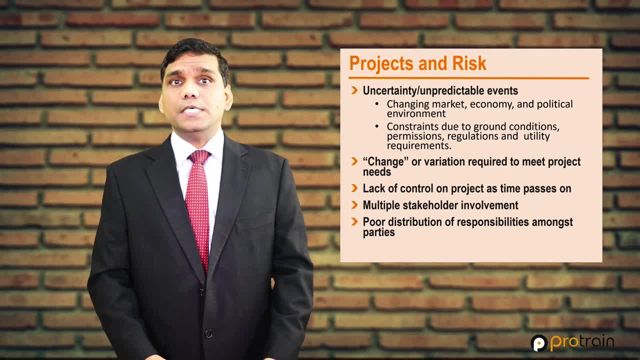 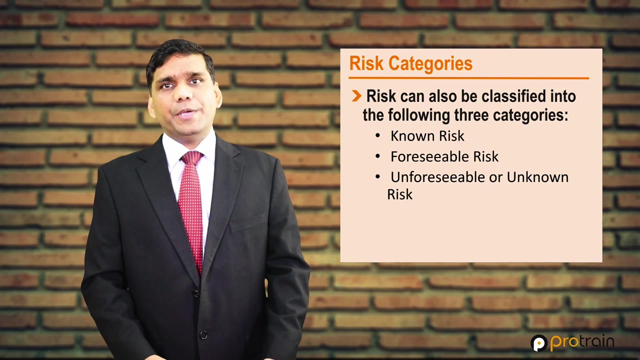 throughout the project life cycle. these variables had some uncertainty, and risk is effect of uncertainty. construction project shares some common variables, so they also share common risk, yet risk treatment is peculiar to each particular project. researcher and academics have identified as many as 100 different type of risk. in practice also, risk can be categorized in many different ways. 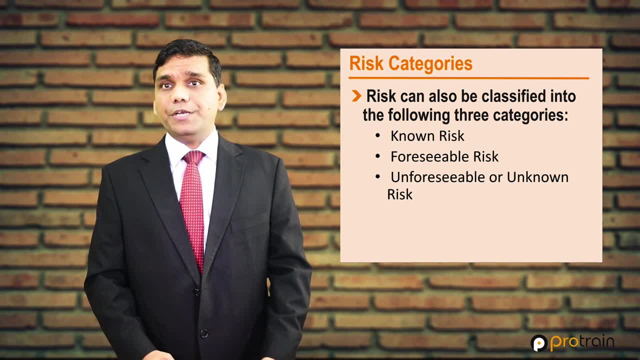 such as known risk. risk are events that have been recognized at the beginning of the project, such as safety risk, weather periods, availability of raw material, etc. for civil risk, on the other hand, a reasonable review should able to identify a risk in a given set of circumstances, for example, availability of 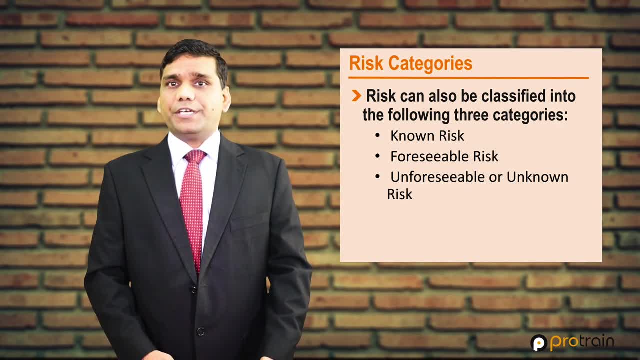 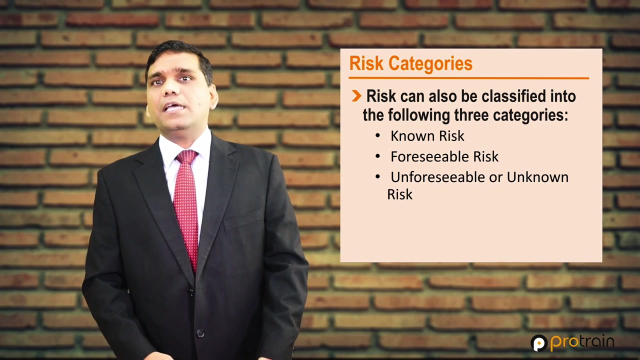 experience. subcontractor in project area or presence of underground cavities could have been identified by review of geotechnical investigation report unknown risk. on the other hand, those events were unforeseen by the project team, such as sudden strike, despite of a stable political and labor environment. while doing the classification, 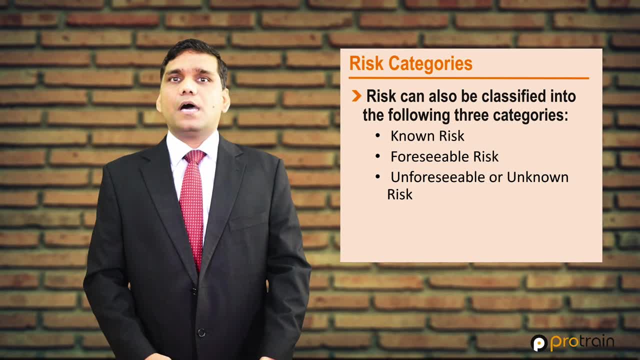 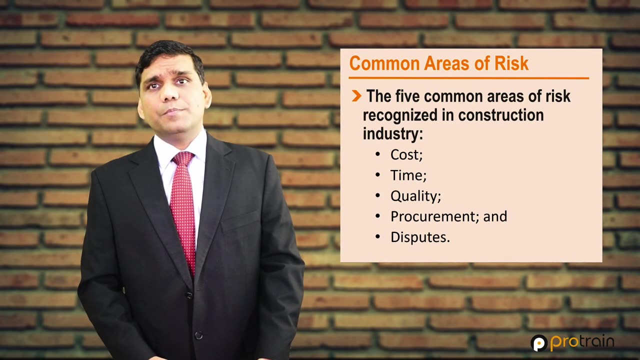 of risk. we need to understand that project risks are separate from the organizational risk. adverse impact on project- that matters and just worry that it happens after the team member or Non-Owner R&D. and another insight is planned leave or any other related tasks, such as resignation of the team members or unpleasant leave by a key person On the project. we have to. 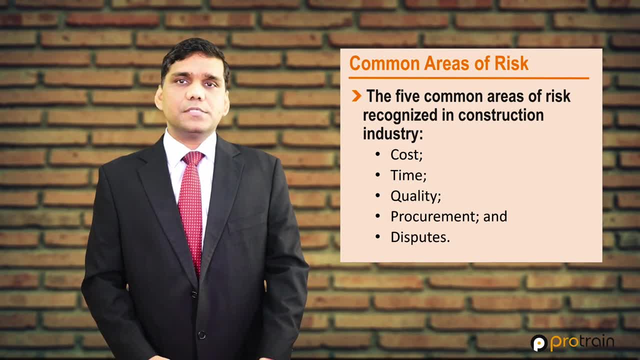 We have to understand that risk perception is generally influenced by people's knowledge, experience, belief, attitude, judgement and feelings. We have to understand that risk perception is generally influenced by people's knowledge, experience, belief, attitude, judgement and feelings. costs- costs- risks- are related to failure to keep within budget forecast, as the policy at all indicates that there is no deeper informat단 to issue management with regard to such risks. 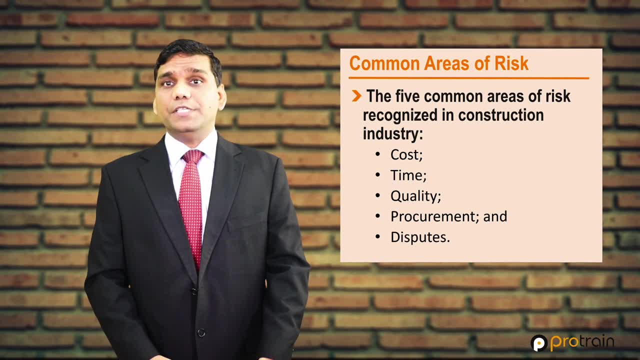 risk perception by the personal people on an individual profit or risk. 여러분들, the understanding of common knowledge, 20 rules, a tier of the risk concepts: estimate, tender. Time-related risks are failure to complete within the time specified or complete the design or commissioning within the allocated time. Quality risks are failure to meet quality. 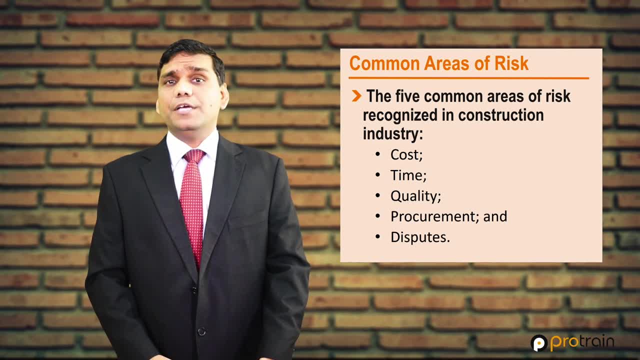 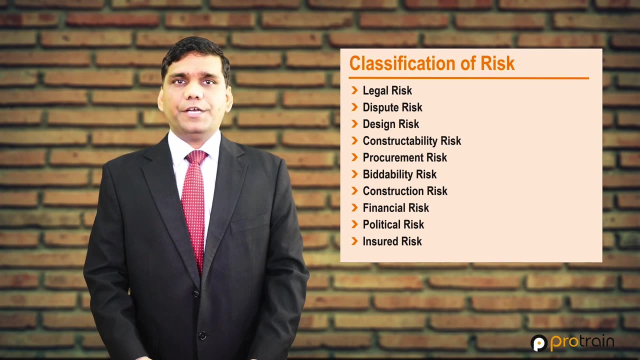 function, fitness for a particular purpose. Procurement-related risks are failure to receive the long lead items, impacting cost and time. both and dispute risk originates from the allocation of the risk in contract form. Let us talk about different kind of risk. Legal risk arise out of: 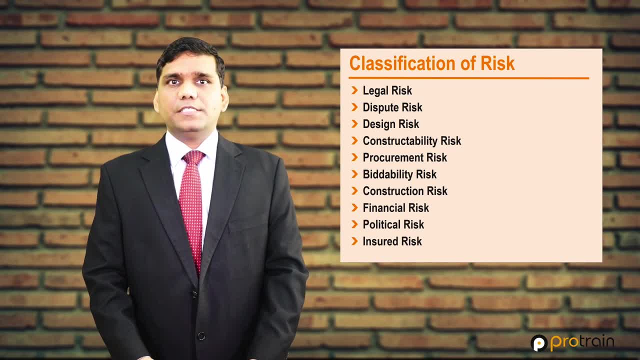 contract is interpreted and legislation enforced, such as environment and related to pollution, etc. Dispute risk arise out of one-sided basis scope contract and delay in settlement of contractors genuine claims. Design-related risks are result of error in design and failure to coordinate design among different disciplines. 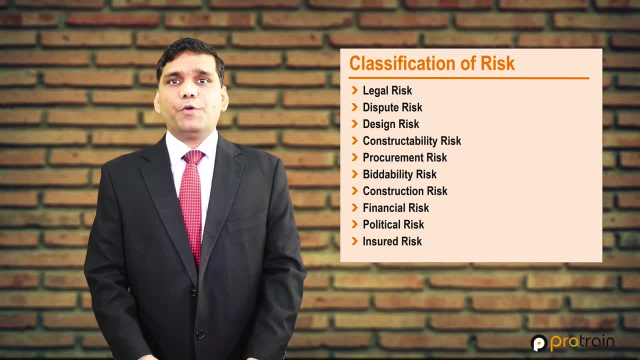 Majority of claims have their bases in defective and deficient drawings, design and specifications. Late finalization of mechanical and electrical details is common risk and cause of delays on project. constructibility Means the ease with which a project can be turned into a final cost. 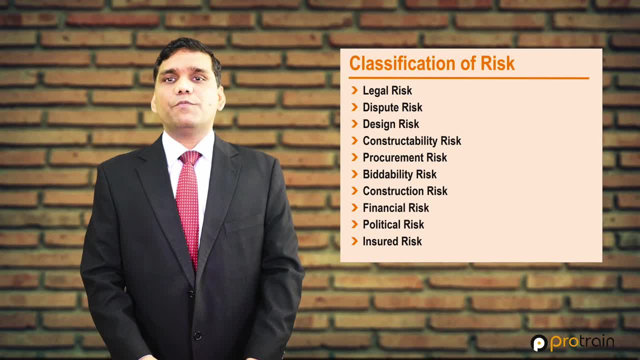 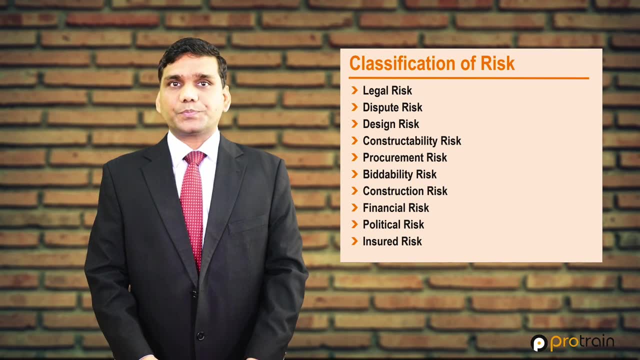 physical reality. These risks arise from site accessibility issues, such as heavy lifts and work-related methodology. Procurement risk relates to the selection of right form of contractor suitable to work in question: One single large contract or separate contracts at work package level? Bidability risk is related to misinterpretation. 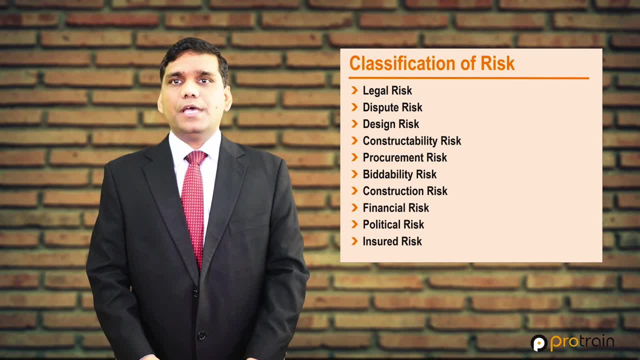 of the tender documents about what is required At the outset of the project, especially in ESPC projects. price expressly includes the things not shown on feed drawings, however deemed to be included in the scope of works to achieve fit-for-purpose works Construction. 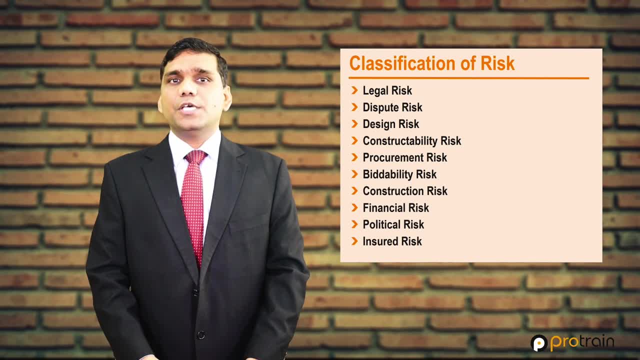 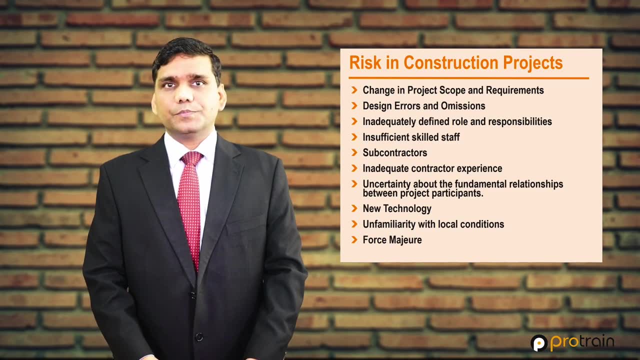 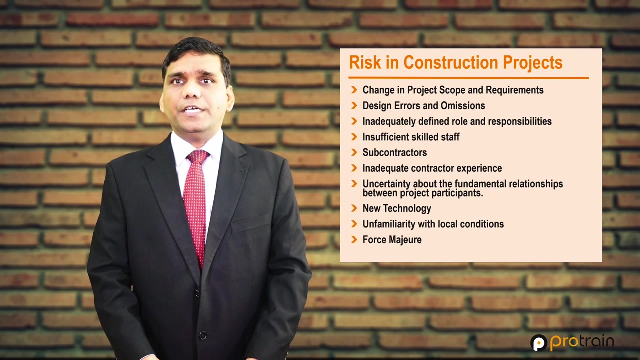 risk relates to change in project owner requirements without extension of time, inclement weather for a long period of time. Generally, risk sources can be divided into external sources and internal sources. The external sources, such as natural disasters, law changes, and internal sources are design. 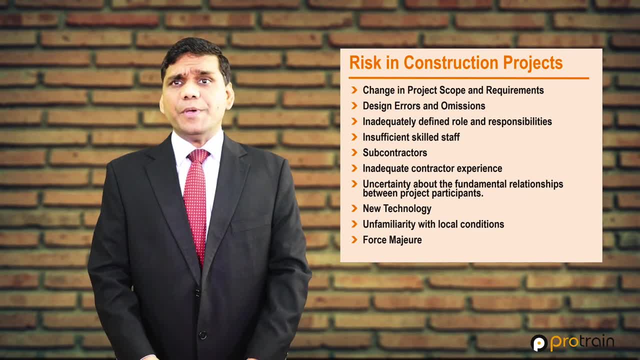 errors. low productivity of subcontractors, Irrespective of it is external or internal. some typical sources of risk are listed below: Change in project scope and requirements. Design errors and omissions. Inadequately defined role and responsibilities. Insufficient skilled staff Subcontractors. Inadequate contractor experience. 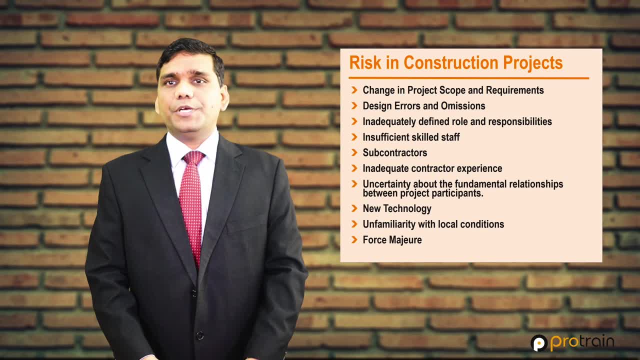 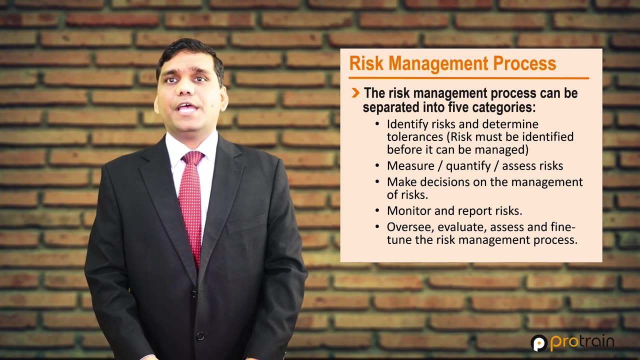 Uncertainty about the fundamental relationships between project participants. New technology, Unfamiliarity with local conditions, Force major Cond прям Disília. it is necessary to have a clear vision of the event. No technological challenge, No kitten death. The matchmaking problem badge and its impact can achieve fixedñana. 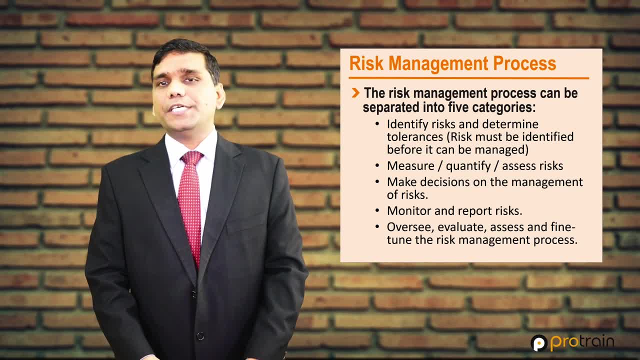 can be accommodated. The second step requires analysis. The success여�ice can be determined by the sequence of processes of the risk, qualitatively and quantitatively. once the risk is analyzed, then it is required to be treated by risk avoidance, risk transfer risk. 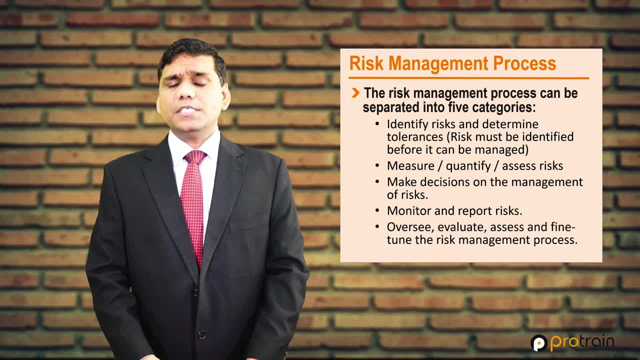 mitigation and risk acceptance. risk avoidance is about not proceeding or eliminating the root cause of the potential problem. risk transfer is possible through insurance to insurance companies, through subcontracting to subcontractor, through modifying the contract terms and conditions to client or other parties. risk mitigation relates to the reduction of probability and our 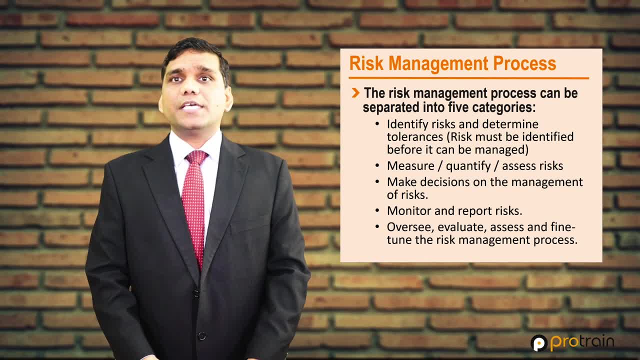 impact of an adverse risk event to an acceptable threshold. taking early action to reduce the probability and our impact of a risk is often not possible. risk management is often more effective than trying to repair the damage after the risk has occurred, for example, verify the site data and perform additional survey to mitigate design related risk. risk management is a continuous process throughout the life cycle of the project and it should not be stopped at any stage. 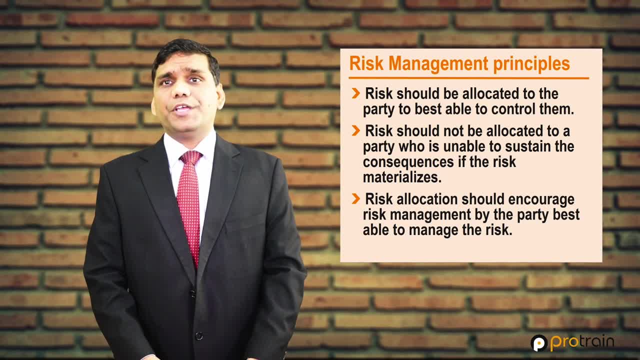 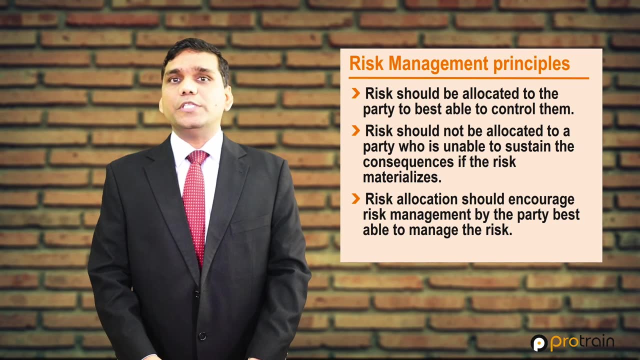 These days, employer are transferring more and more risk on to contractor in design and build projects, while missing the basic point that risk should be allocated to the party to best able to control them. I hope you like this short presentation on risk management in construction projects and we will come. 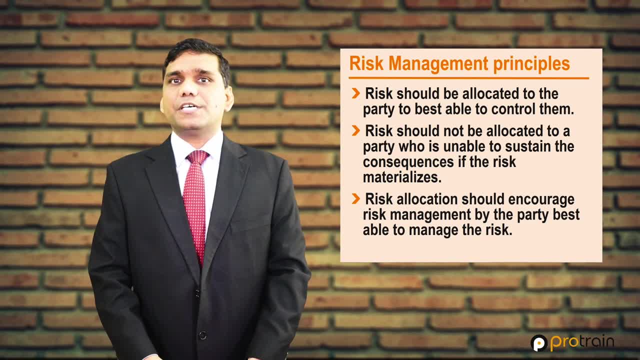 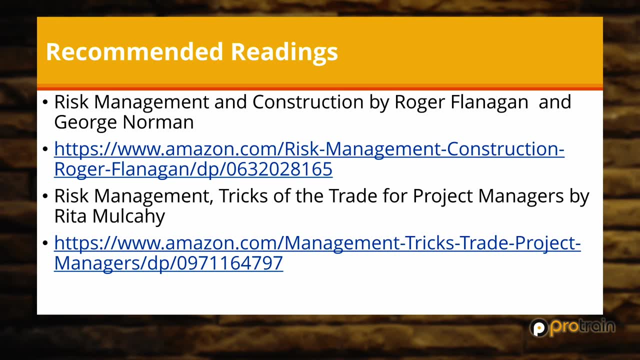 back again with risk analysis and risk mitigation strategies in our next video. you may refer these additional resources for further reading and analysis, which are shown in the description of video links.